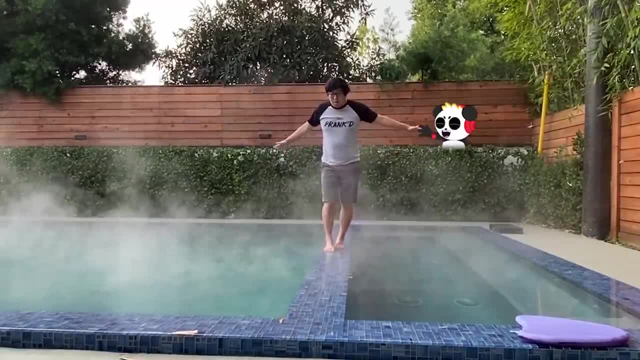 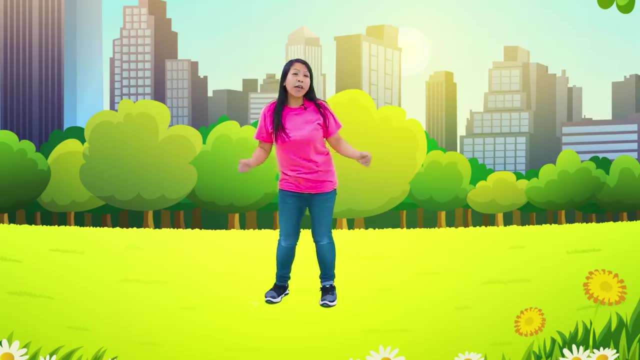 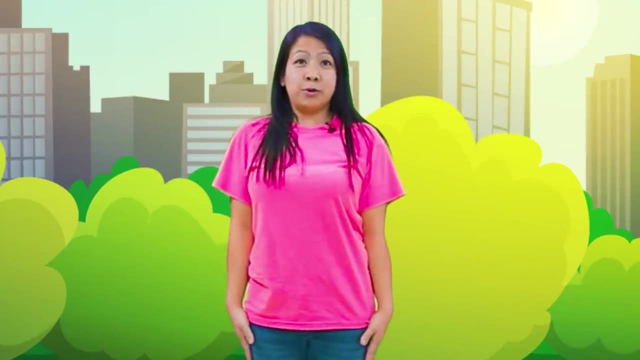 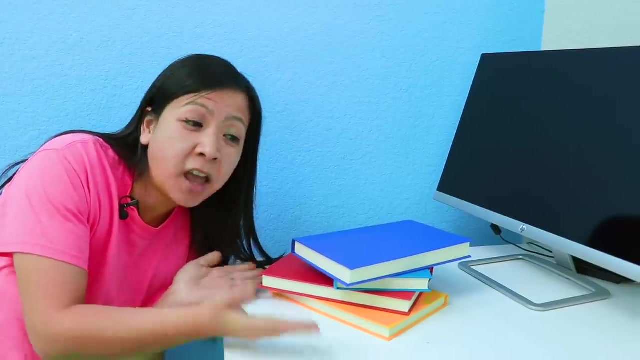 When Daddy fell into the pool. Hey Sean, He is also in motion, Uh-oh. So if motion means moving, something that is not in motion means it's at rest. Here, books are on a desk, They are at rest. 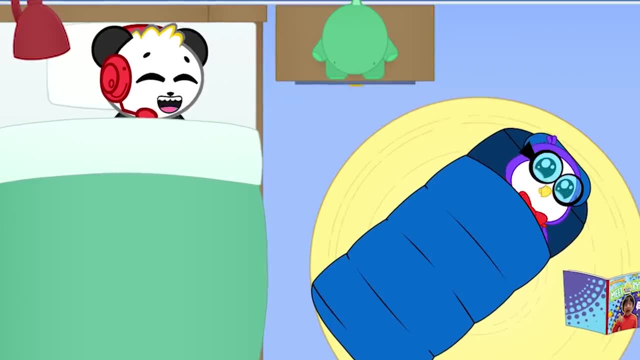 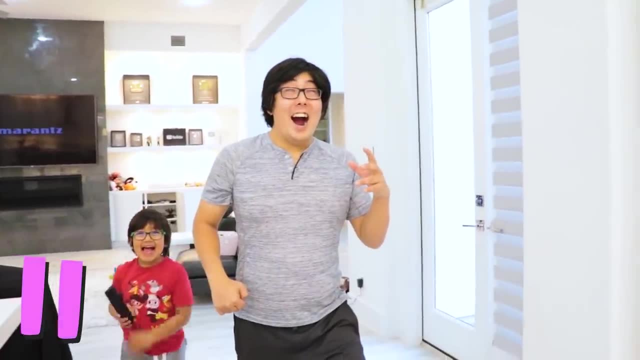 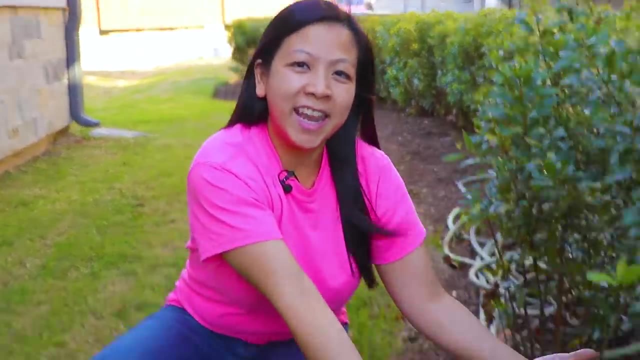 Here Combo is sleeping. He's at rest. Now Ryan paws Daddy. So Daddy is not moving. That means Daddy is at rest. Why, Daddy, are you going so slow Here? rocks are just sitting outside. They are at rest, Not in motion. 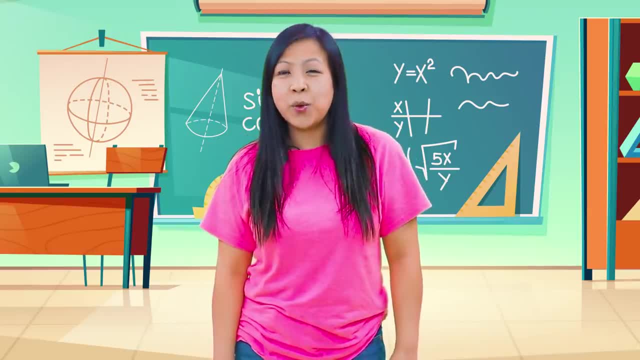 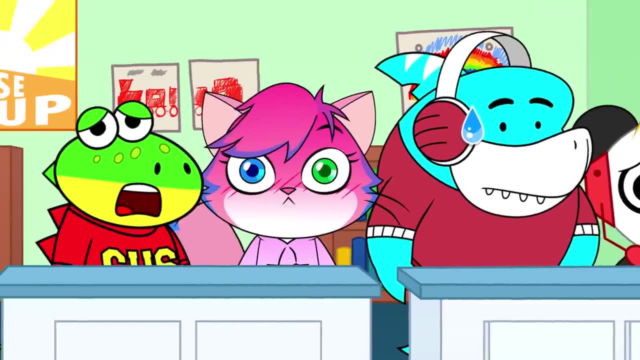 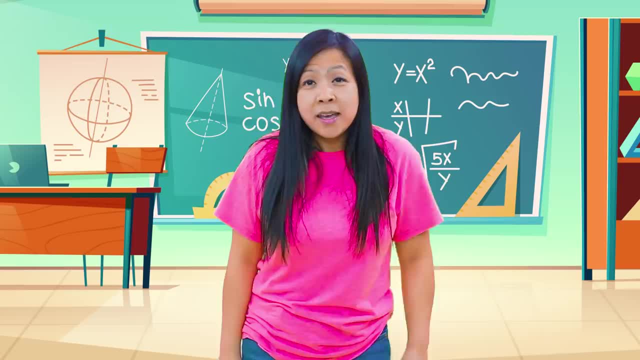 Alpha Me Me Me Me Me Me Me Gus. Hey Me Me Me Pe. Peck, you look like you have your hand up Force, That's right. Good job, Peck, It is FORCE. 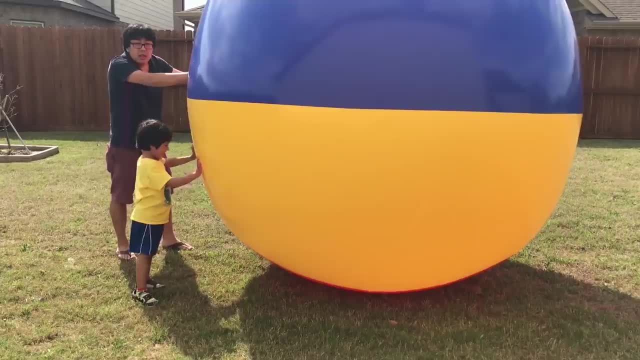 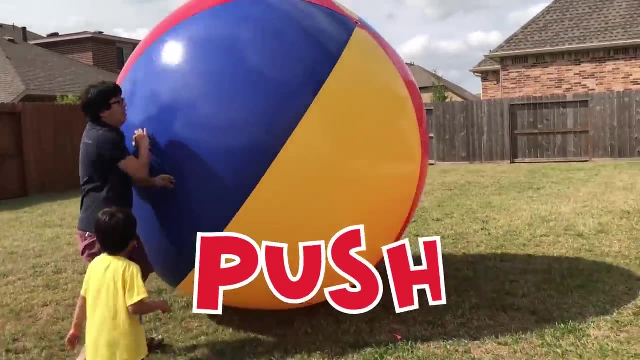 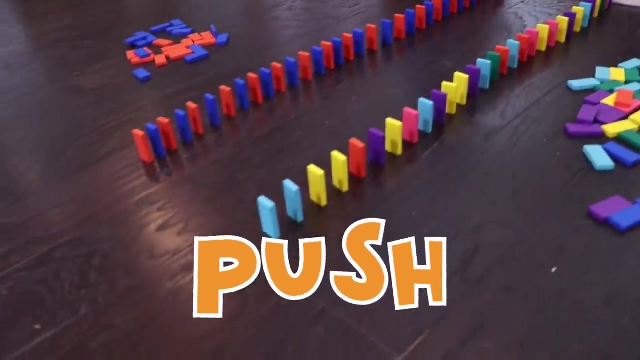 A force is a push or a pull. For example, here Daddy and Ryan both use force, a push to move the giant ball. Here Daddy and Ryan both use force, a push to move the giant ball. Here Ryan uses force, a push to knock down the dominoes. 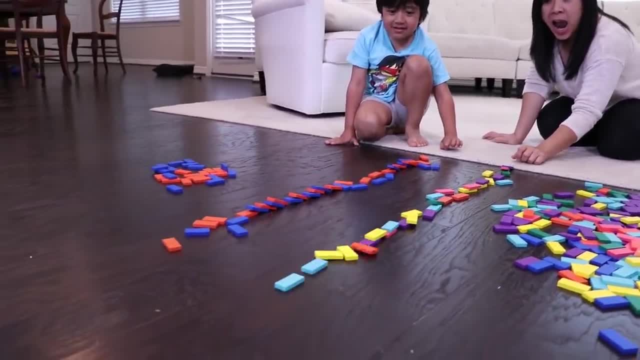 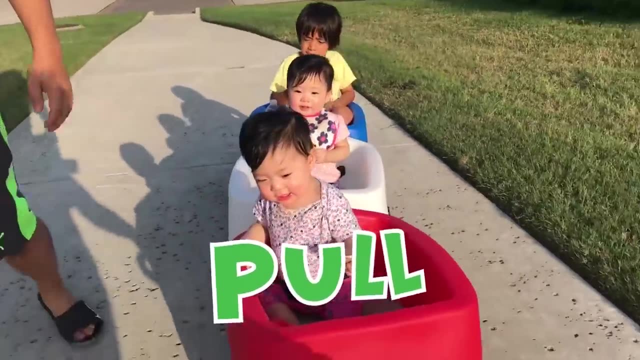 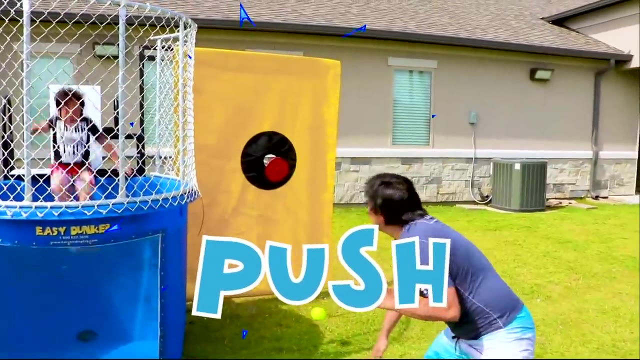 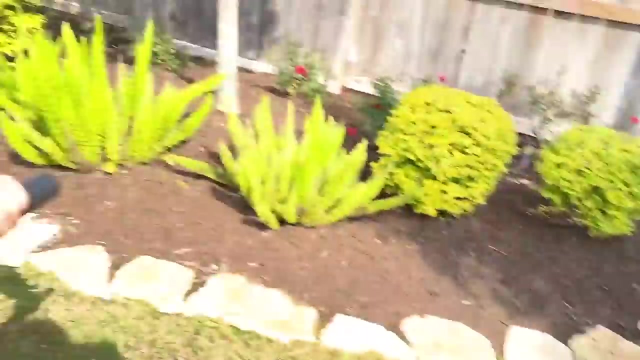 Daddy uses force to pull on the wagon to take Ryan, Emma and Kate for a ride. Daddy also uses force- a push of the ball- to hit the target and Ryan went into the water. Here Emma and Kate both use force to push and pull each other up and down the seesaw. 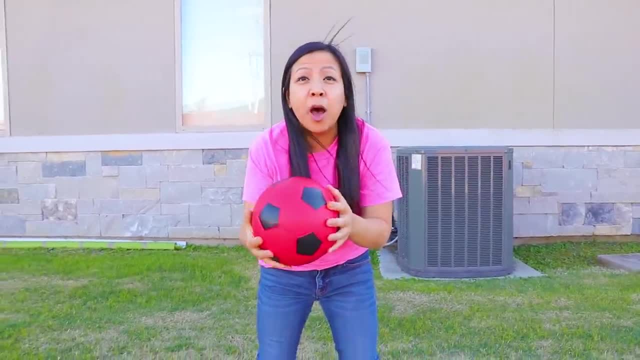 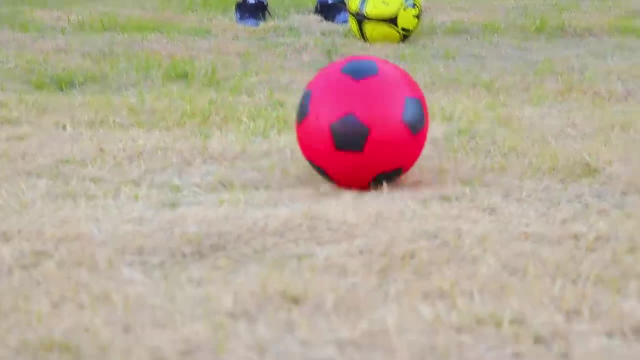 When you kick the ball, you place force on the ball which makes it move. Let's look Here. it is a little force. The amount of force you place on the ball makes a difference. Watch, Okay, here's the ball. 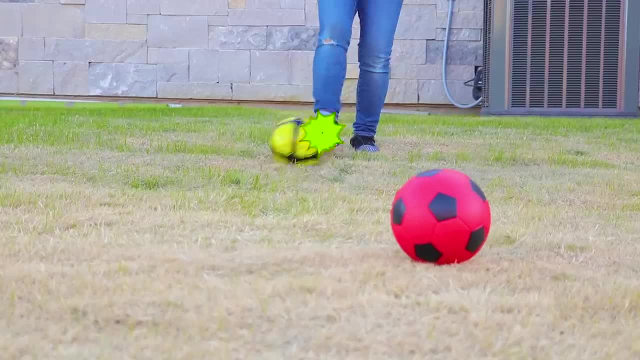 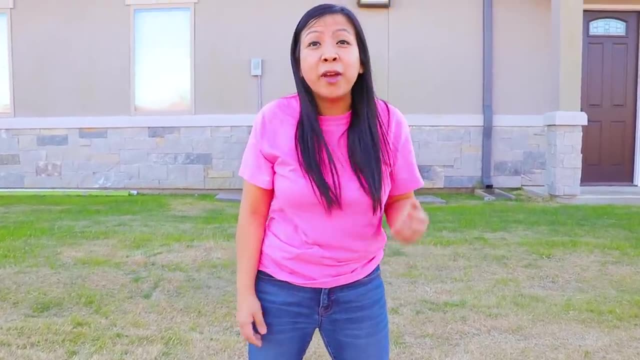 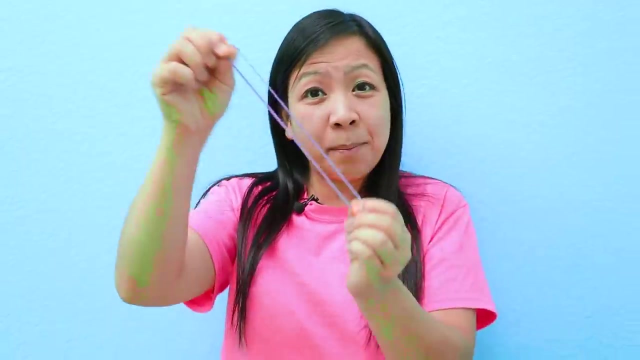 I'm going to use greater force. You guys ready? Say yeah, Yeah, Yeah. Since I put more force on the green ball, it went further than the red ball. look, A rubber band is also a good example of force. 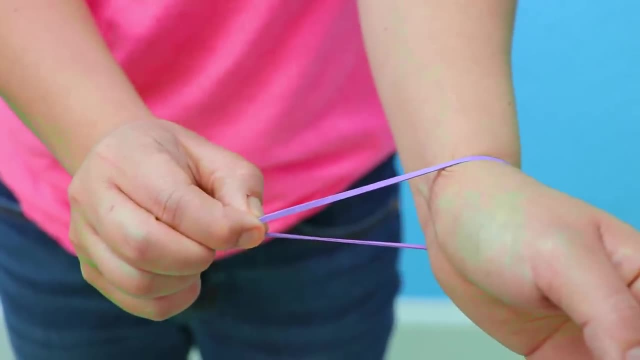 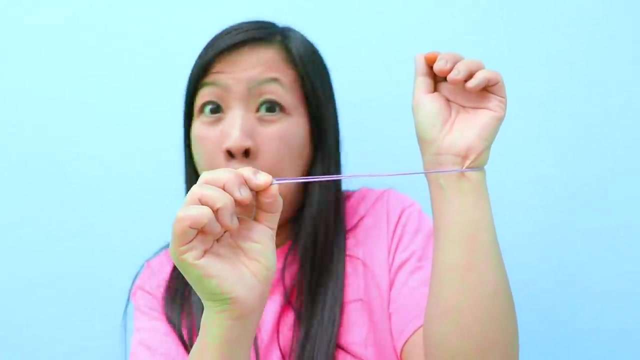 When you pull on a rubber band, the force that you pull will come back at you, But be careful not to use too much force Using force. let's make a swing shot Using a rubber band. First, fold the small paper like this: 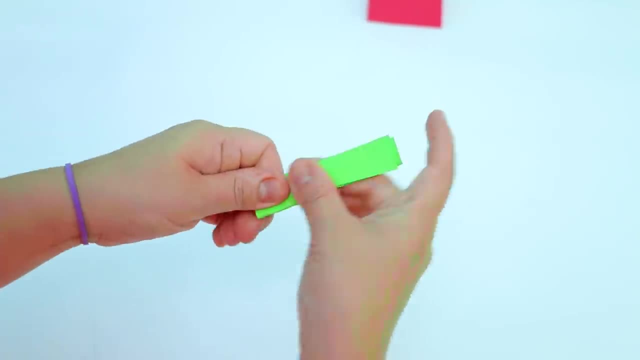 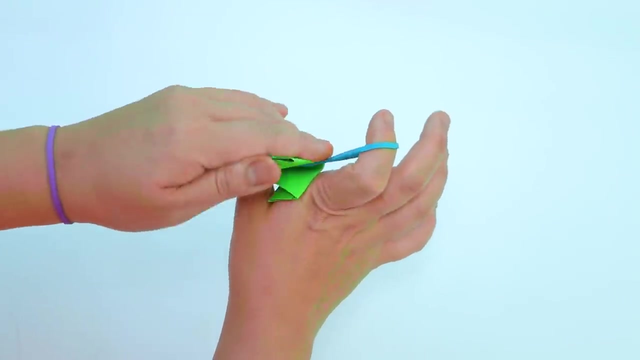 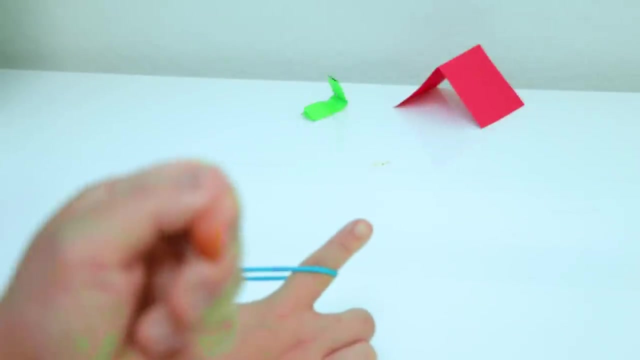 Then fold the paper on top of the rubber band, Pull with enough force to launch the rocket and knock down the goal Score. So let's recap: An object could be in motion or it could be at rest. Using force, let's make a swing shot. 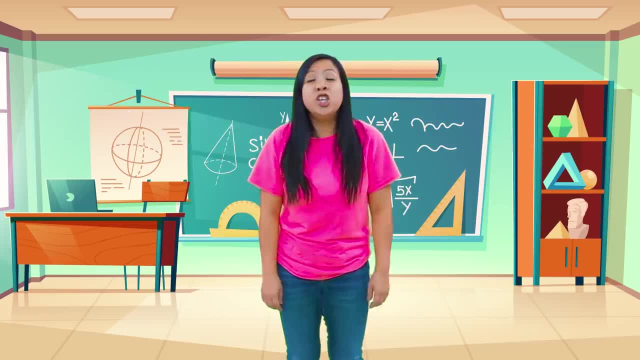 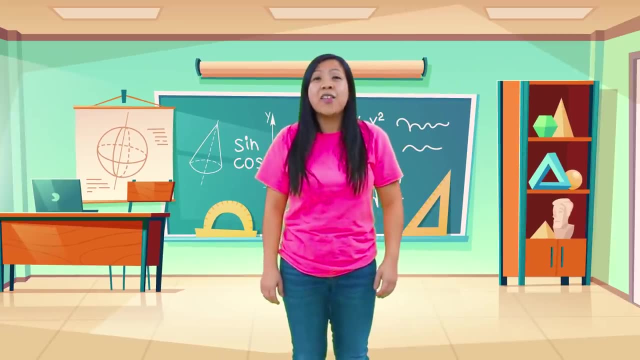 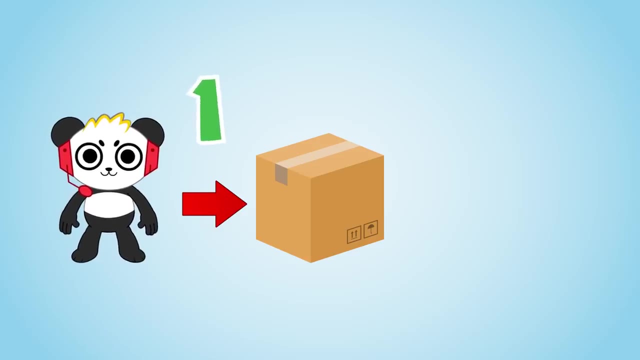 Using force. let's make a swing shot Using a rubber band. First, fold the small paper. like this, Using force, which is a push or a pull, you can put an object that was at rest in motion. Combo uses a force of one, while Alphaluxa uses a force of three. 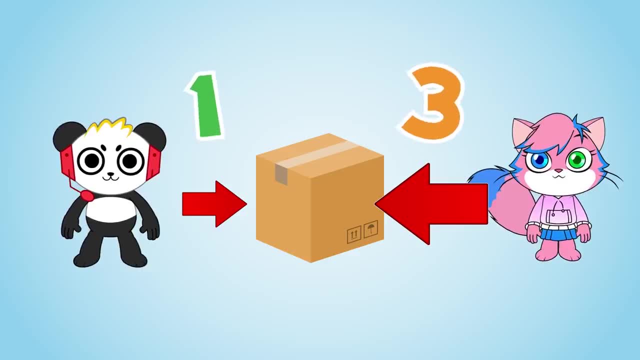 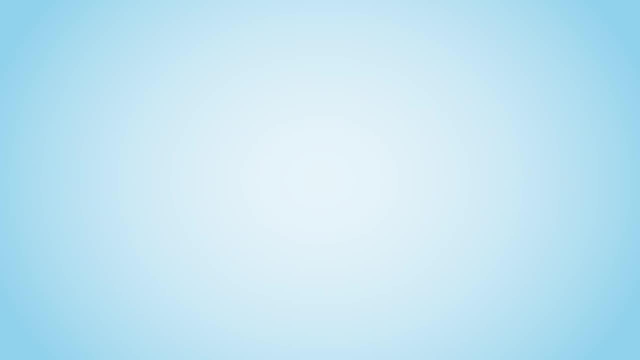 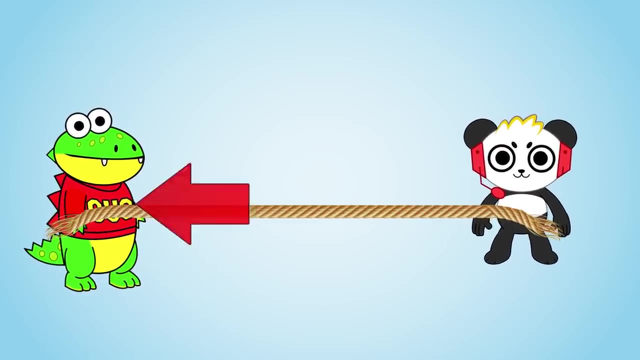 Which way will the box move? That's right towards Combo. The greater force will put the box in motion. Let's try another example. Gus and Combo are playing tug-of-war. Gus pulls with a force of two, Combo also pulls with a force of two. 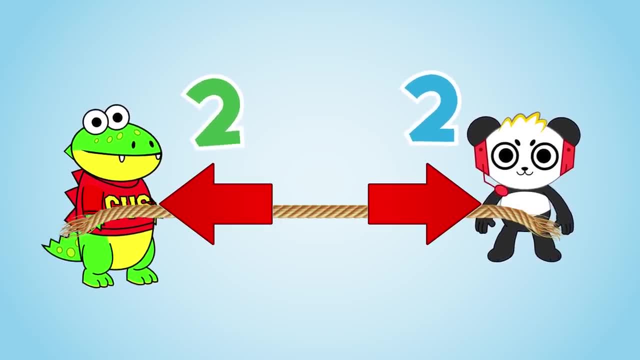 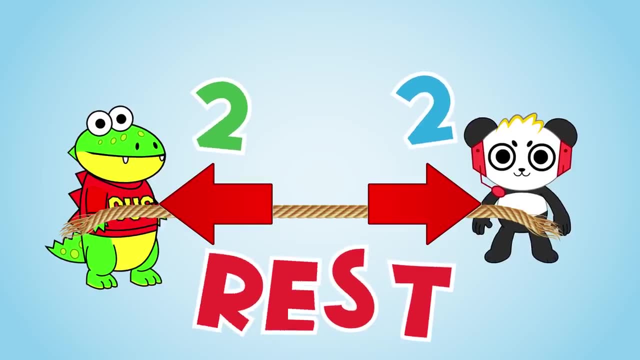 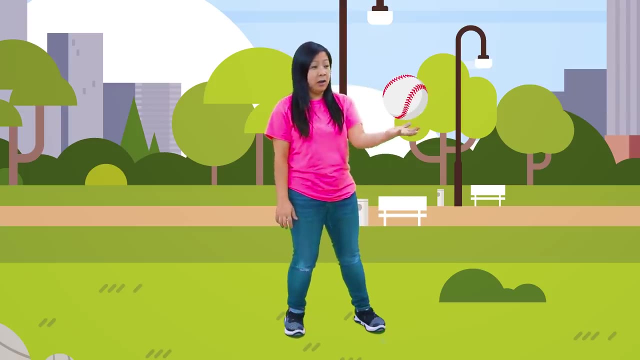 Since they both pull with the same amount of force, the object will not move. It will remain at rest. Greater or stronger force may cause faster motion. Look, I'm putting a lot of force. Whoa, look at it go. This means that force does not always cause movement. 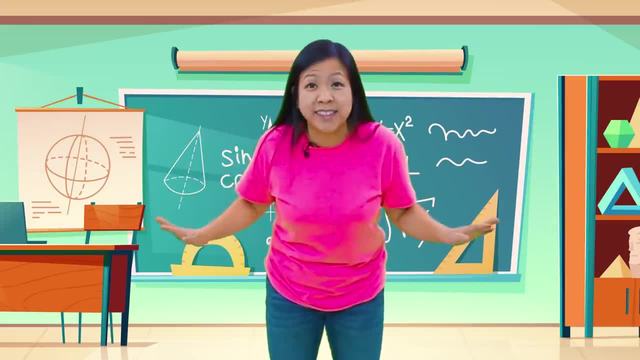 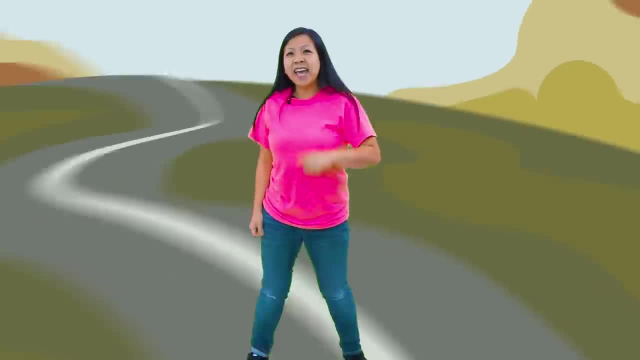 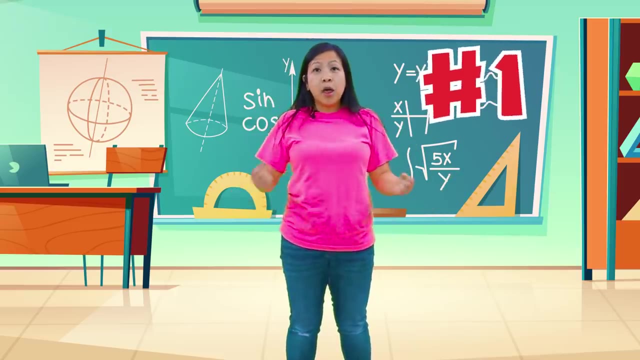 Balanced forces does not cause motion. Now that you know all about force and motion, time for a quiz. Question number one: Which one of these, Which one of these, is an example of motion? Combo Panda Skateboarding- Yeah, I got it. 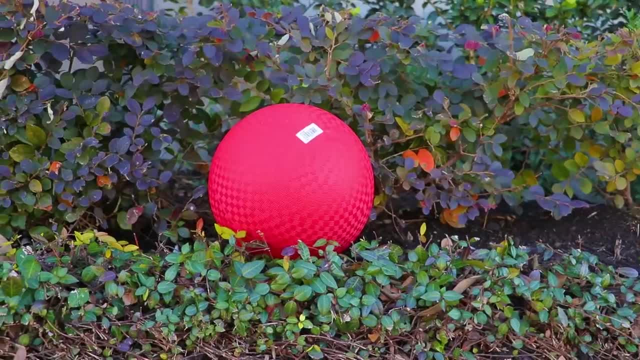 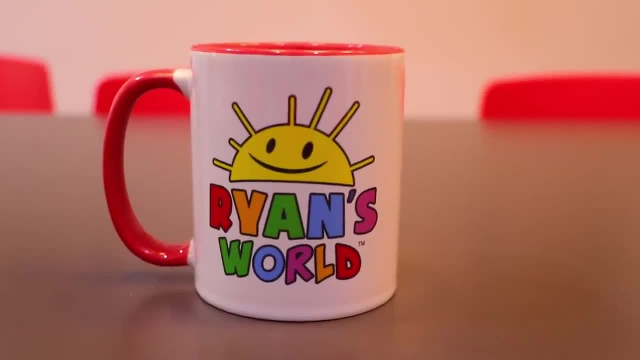 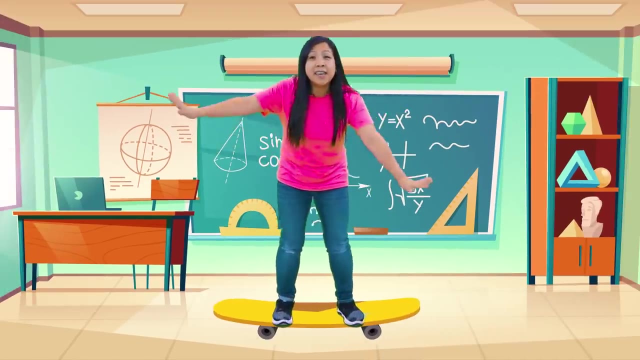 Yeah, Combo Bunga, I did it. Woohoo, A ball sitting outside A cup on top of a table. That's right. the answer is A Combo Panda Skateboarding. He was in motion. That means he is moving. 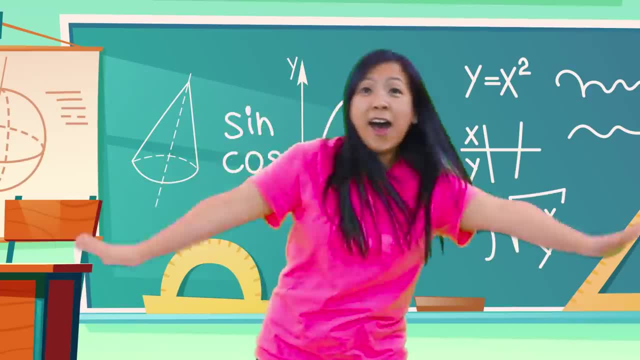 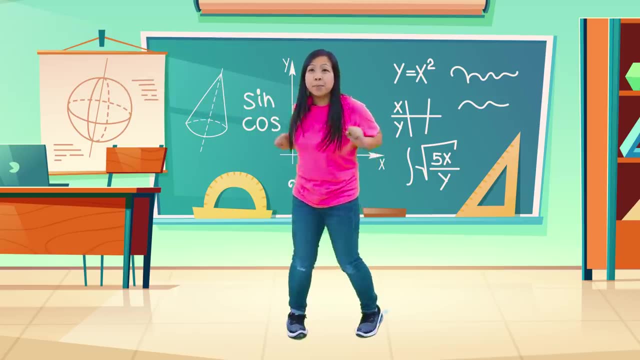 That means he is moving. Whoa, Ah. Question number two: What is the word that means a push or a pull? Is it A peekaboo, or is it B force, or is it C spaghetti? Did you get that? 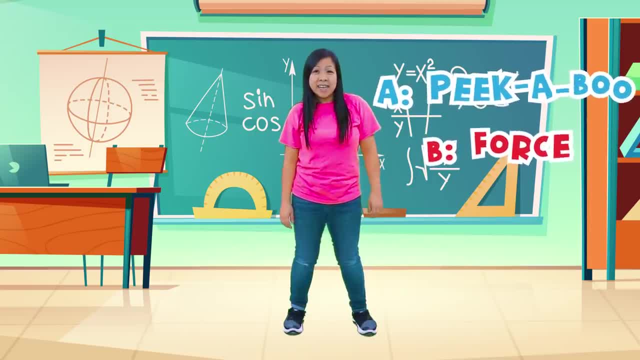 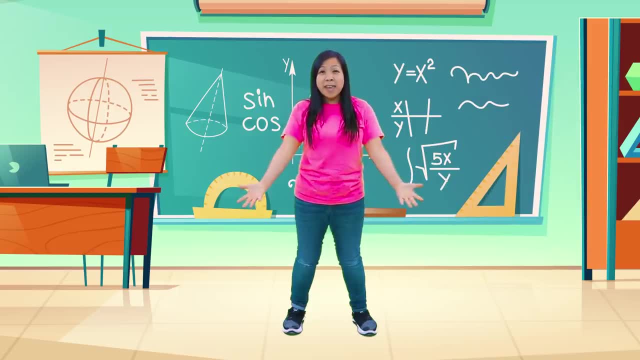 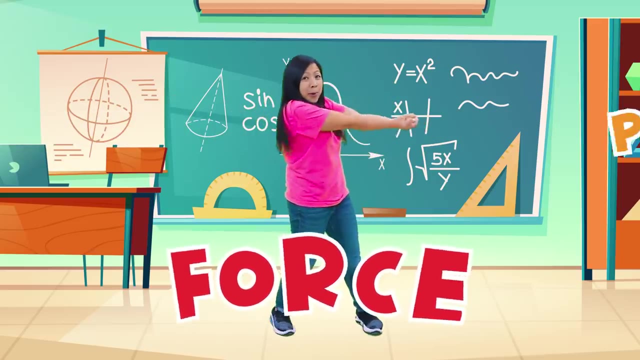 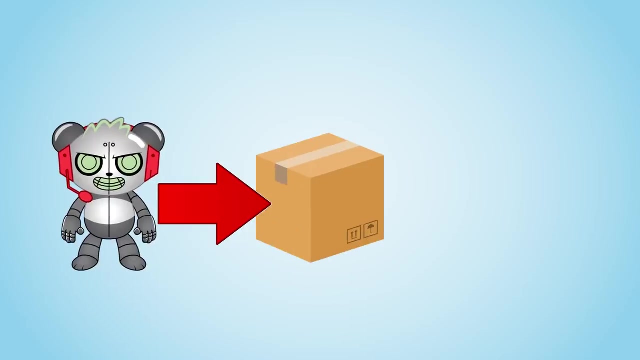 What does it mean? Four, Four, Four, Four, Four, Four, Four. Did you get it? It is B force. A force means that it's a push or a pull. Question number three: If Robo Combo pushes a box with a force of two, 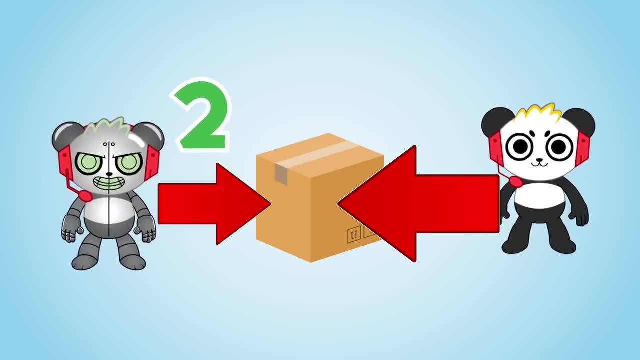 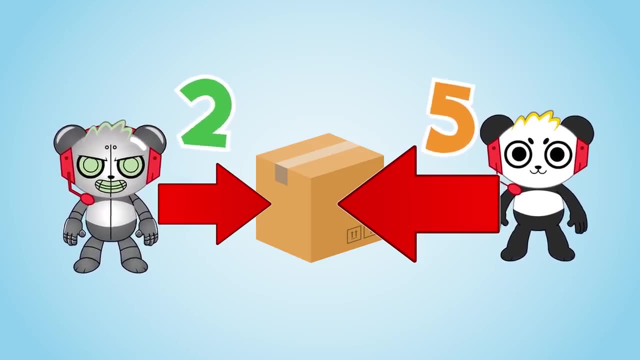 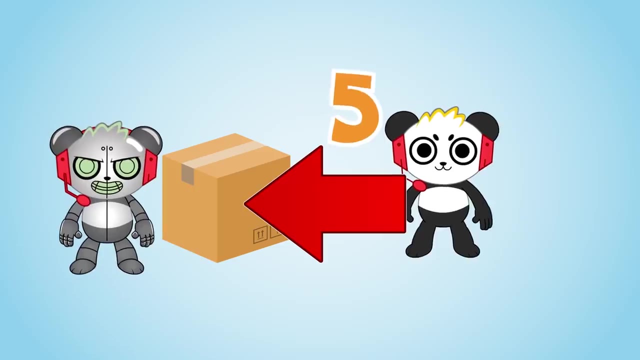 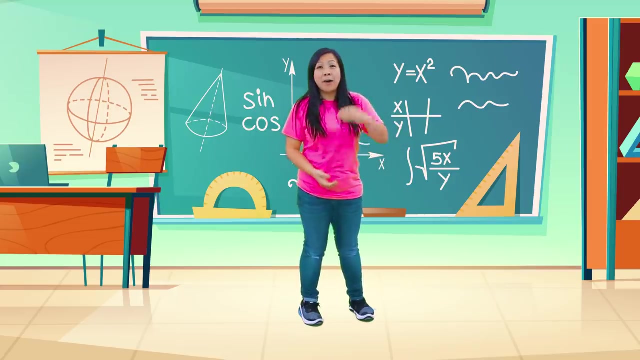 and Combo pushes the box in the opposite direction, but with a force of five. which way will the box move? That's right towards Robo Combo, because Combo's force is greater. Okay, so now we learned all about forces and motion. Let's go back and tell Ryan: let's go. 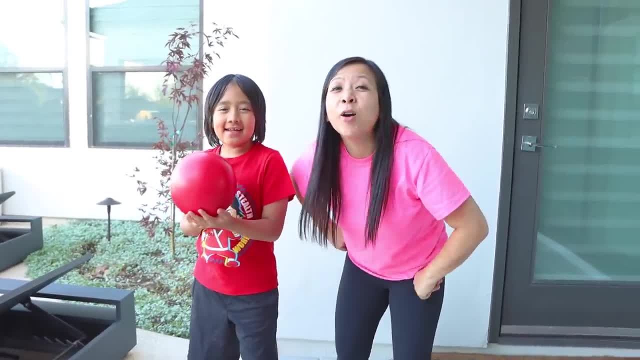 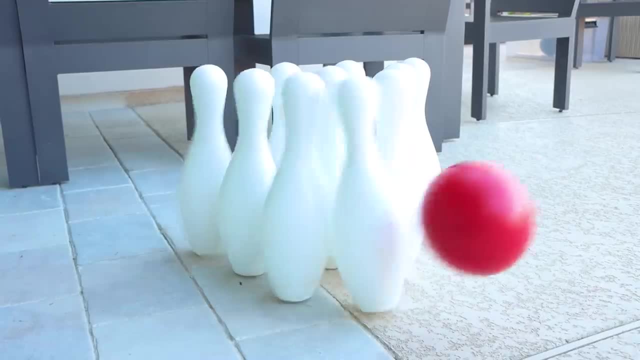 Okay, guys, I'm gonna pull. So, Ryan, that's everything you need to know about force and motion. Yeah, I'm gonna use my hands, I'm gonna use my force right now And I'm gonna put this ball in motion. 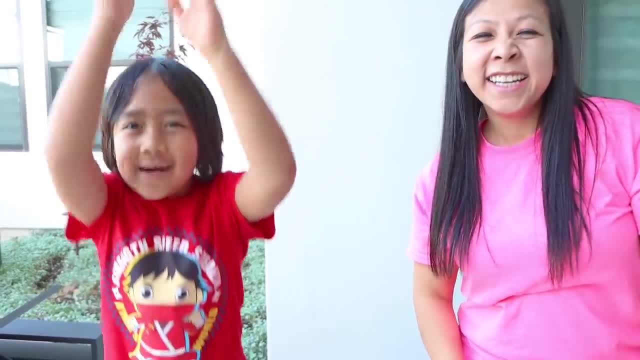 Strike. Thank you for watching. Remember always: stay happy and rise up. Bye Ryan, I'm gonna put forces on you.